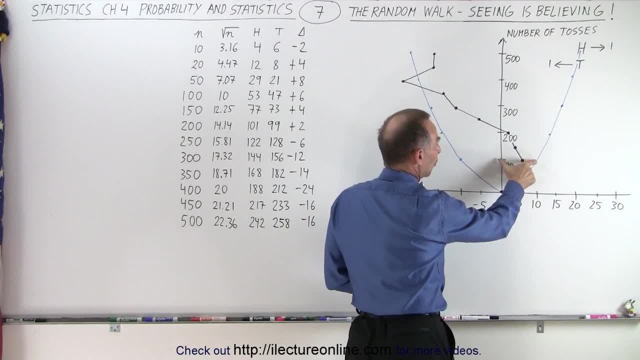 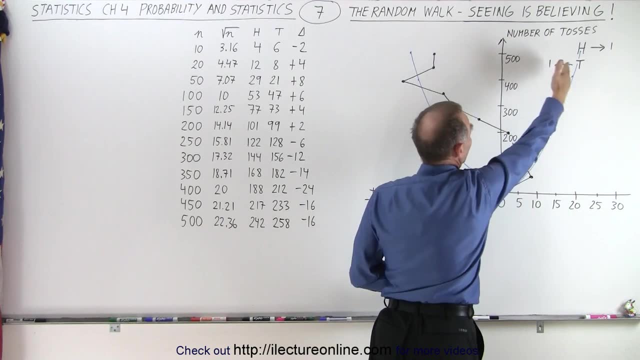 100 tries, you would be 10 steps away, or 10 units away from the origin. After 20 tries, you'd be 20 units away from. after 400 tries, you'd be 20 units away, and so forth. So it would. 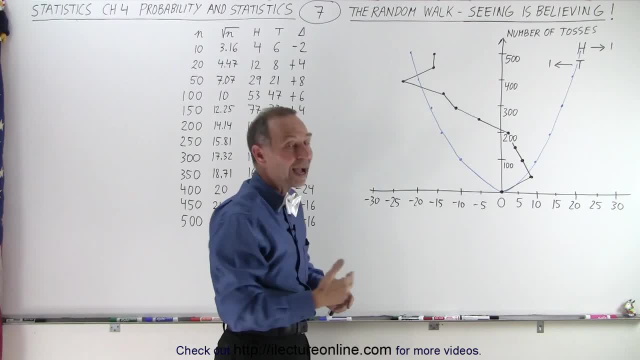 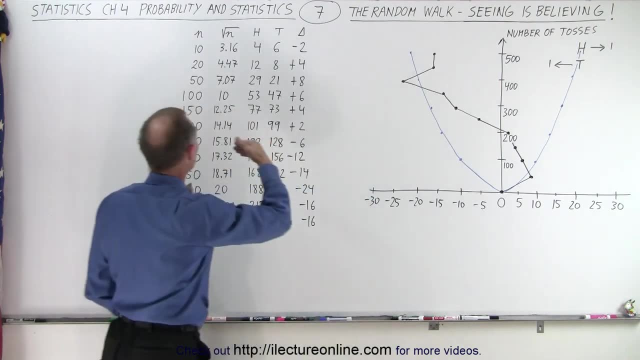 seem like you would be farther and farther away from the origin the more times you toss the coin. So I started tossing and of course we don't have an exact account Counting above 500, I started grouping it. After 10, I ended up with six tails and four heads. 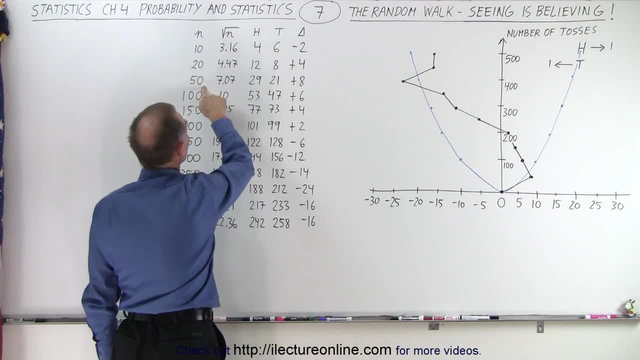 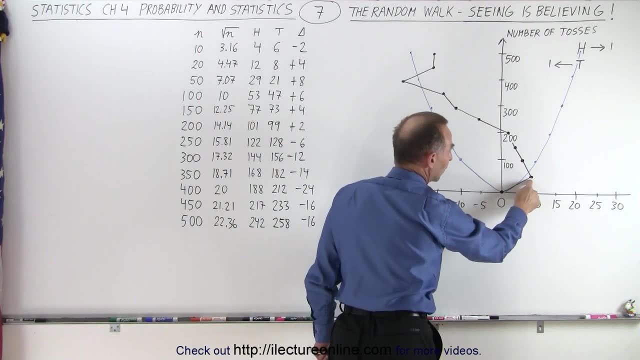 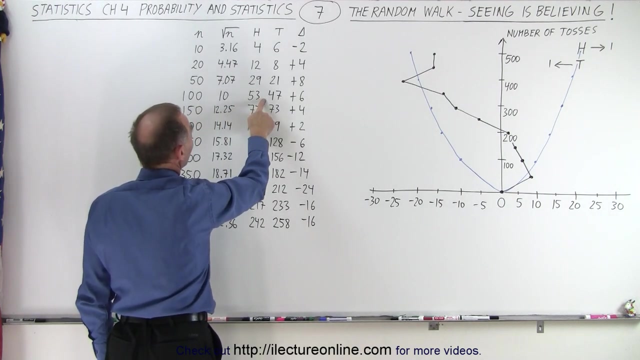 so that's two units to the left. After 50 tosses I had 29 heads and 21 tails, so it was eight units to the right. So after 50 tosses I was over here and it looked like the theory seems to be correct. After 100 tosses I had 53 heads and 47 tails. 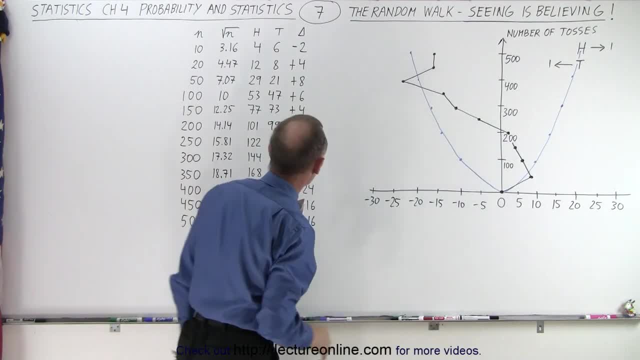 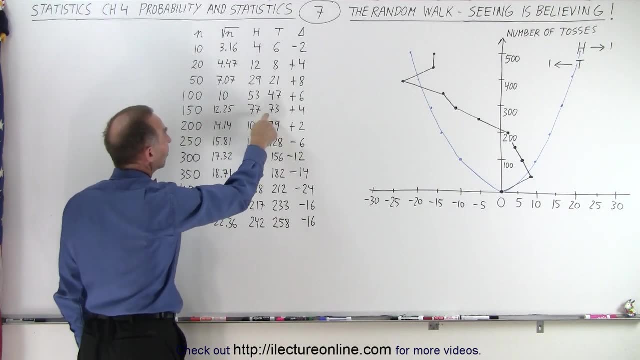 so it was still six units to the right. So it seemed to be following pretty well what it was supposed to. But then 50 tosses. I was over here and it looked like the theory seems to be correct. Things seemed to go kind of strangely. After 150 tosses I had 77 heads and 73 tails. I was only 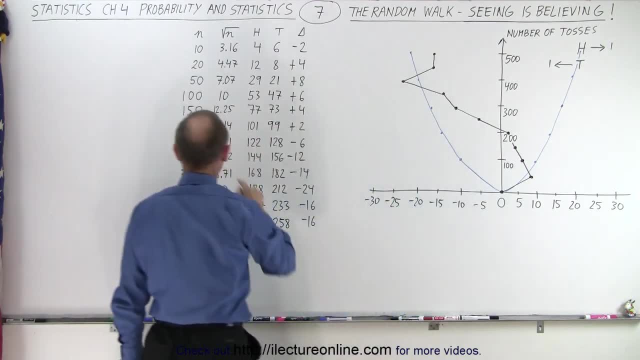 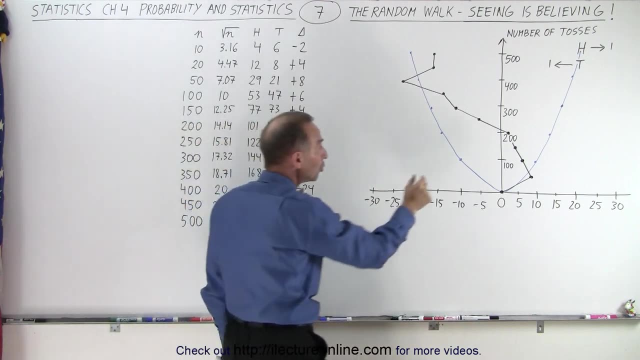 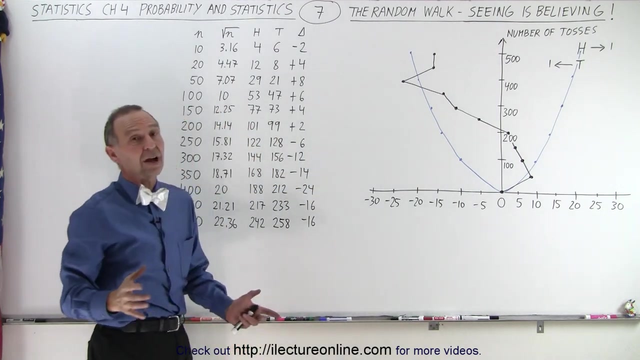 four units away from the origin And after 200 tosses I had 101 heads and 99 tails and I was almost back where I started, only two units away from the origin. So it really looked like that theory of the random walk didn't make any sense. But 200 tosses, even though it's a lot of work. 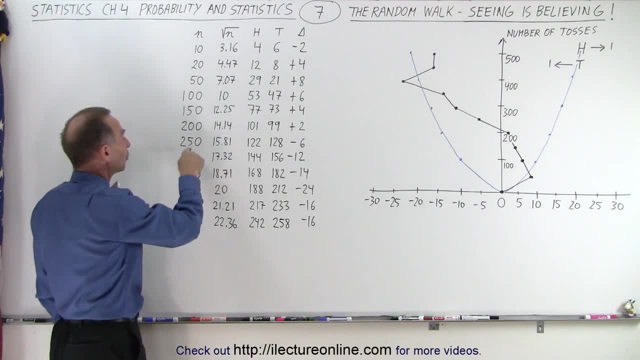 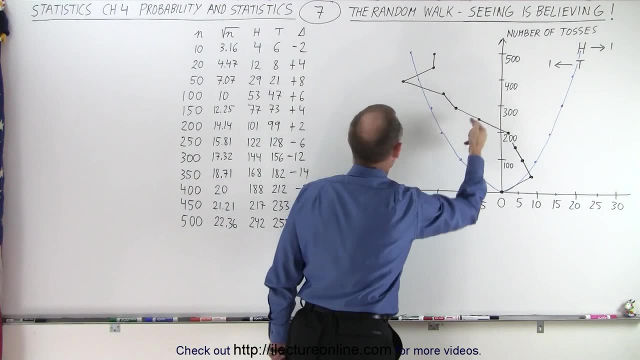 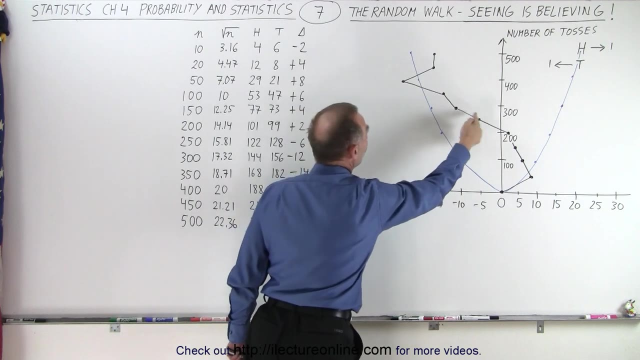 isn't really that many tosses. So as I continued and got up 250 tosses, I had 122 heads and 128 tails and now I was six units to the left. After 300 tosses, I had 144 heads, 156 tails and now I have 12 units to the left After 350 tosses. 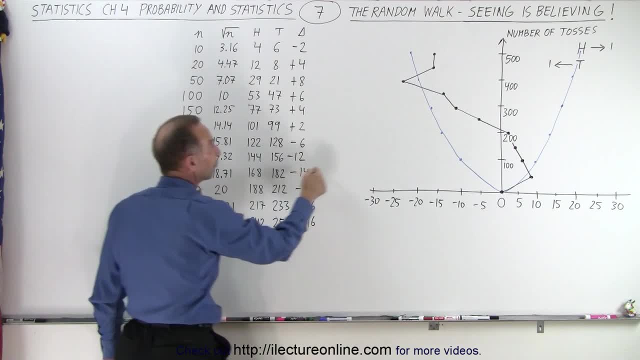 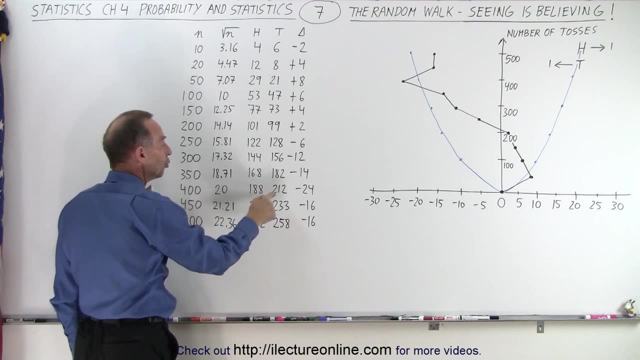 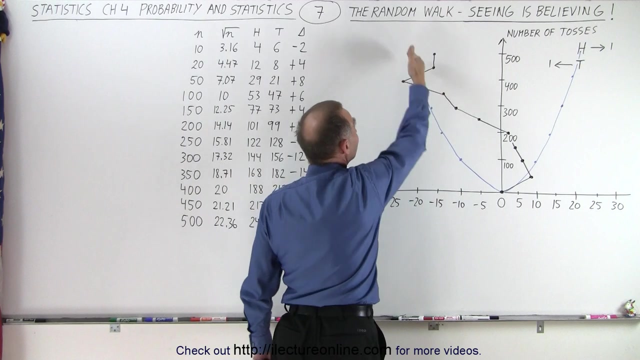 I had 168 heads and 182 tails. I was 14 units to the left. And look at this: After 400 tosses I had 188 heads, 220, 212 tails and I was 24 units to the left. I was well beyond the predicted number. I would. 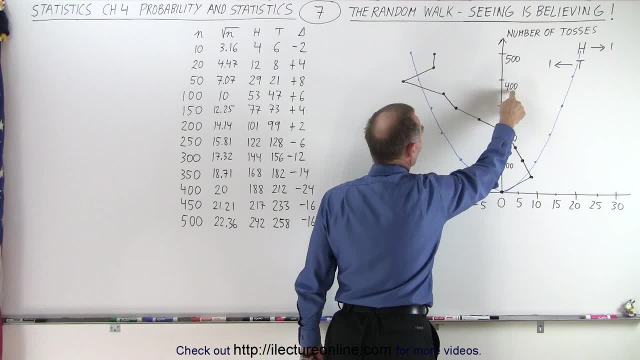 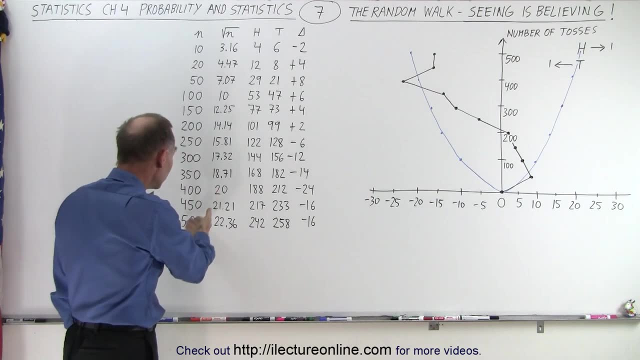 expect, because when we take the square root of 40 or 400, I should get 20, and I was actually 24 units away from the origin. then, as I continued to toss all the way up to 500, then I was only 16 units away from the origin. but you can. 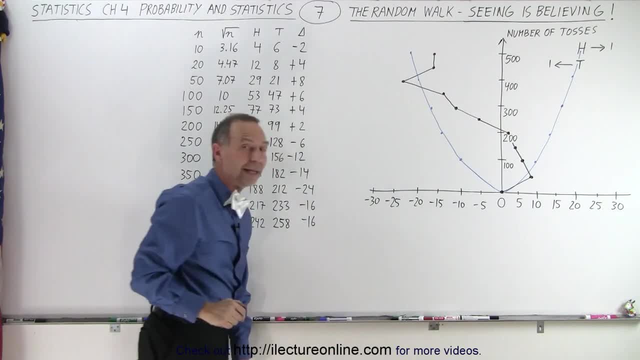 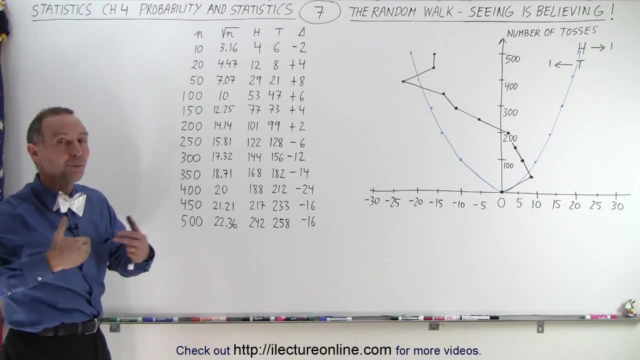 see that I was fairly close to predicted value. it does seem to be the case. you can try this at home. it's kind of fun if you have some time, and you'll see that every time: the more times you toss on average, the farther away you're going to. 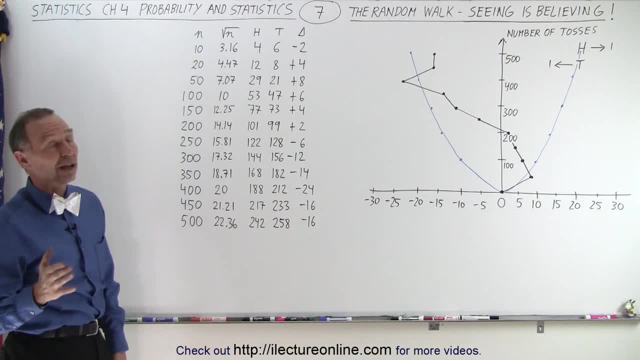 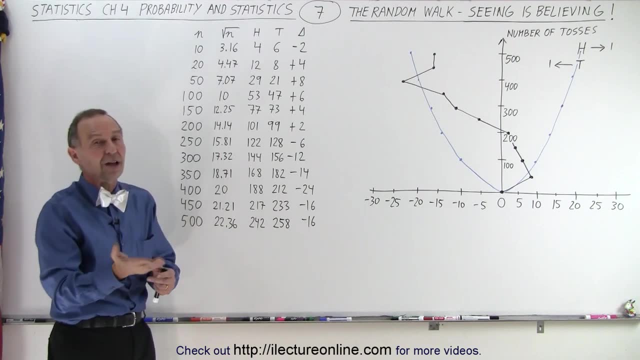 be from the origin, and it will be like that every single time. all you have to do is toss coins enough times or use a die, for example. if it's, if it's even, go one direction. if it's odd, go the other direction, and again you will deviate. 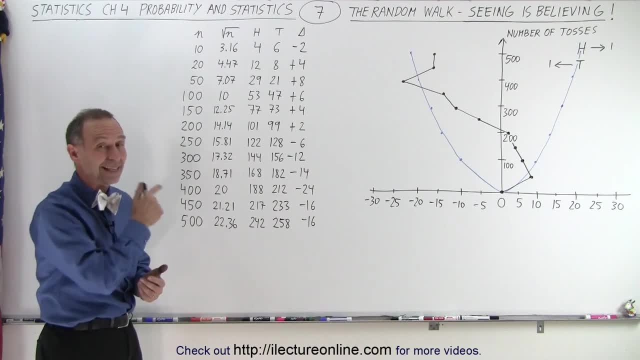 away from the origin if you throw it enough times. seeing is believing. that's the way it works you. 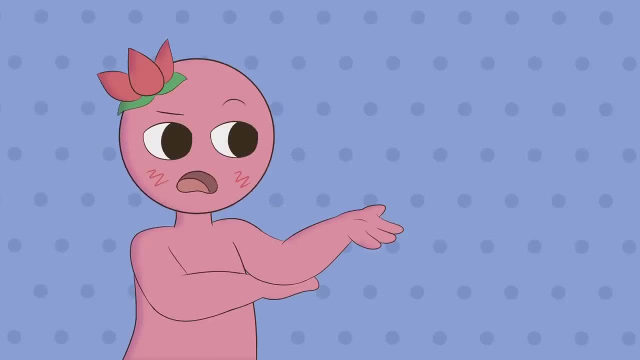 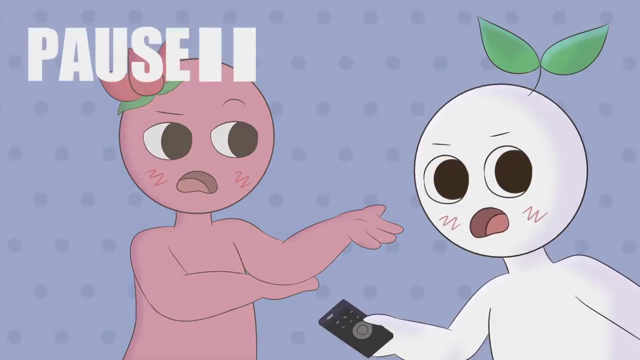 But you were so young when that happened You hardly even remember it. How can it even affect your personality now? Saying things like these cannot undermine the fact that childhood trauma exists, And even if you don't exactly remember it, it still leaves an impact on you. 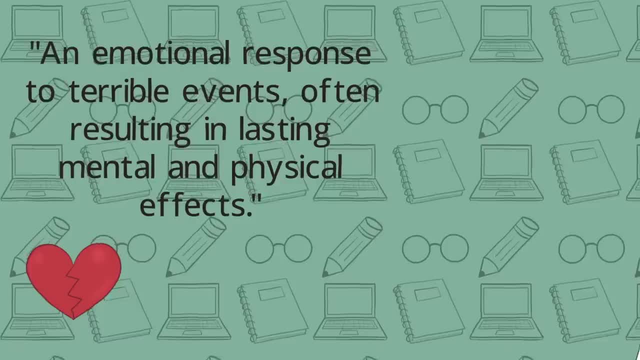 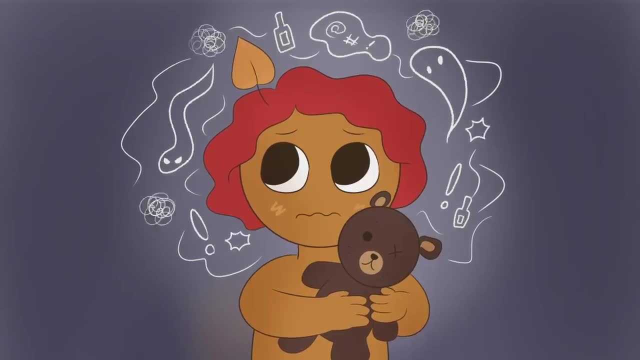 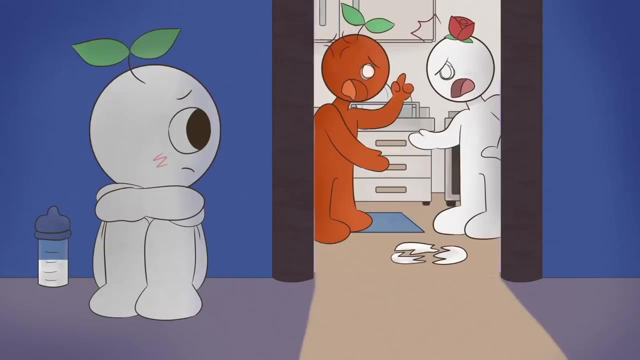 The American Psychology Association defines trauma as an emotional response to terrible events, often resulting in lasting mental and physical effects. Childhood trauma can occur when a child witnesses or experiences overwhelming negative events. This type of trauma falls within the category of interpersonal trauma, which means trauma that happens between people. 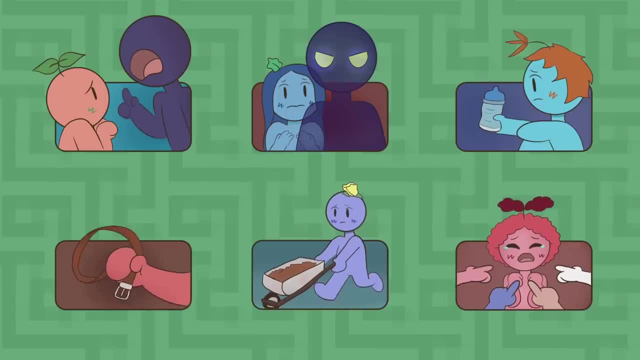 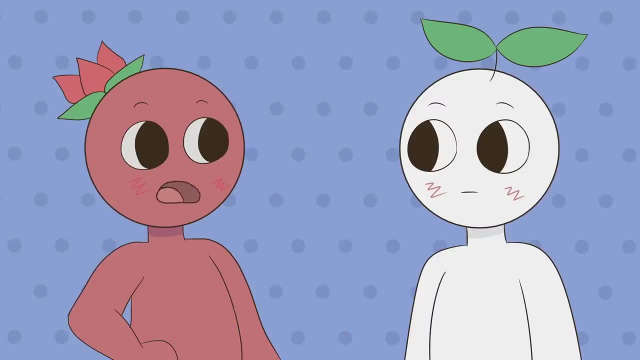 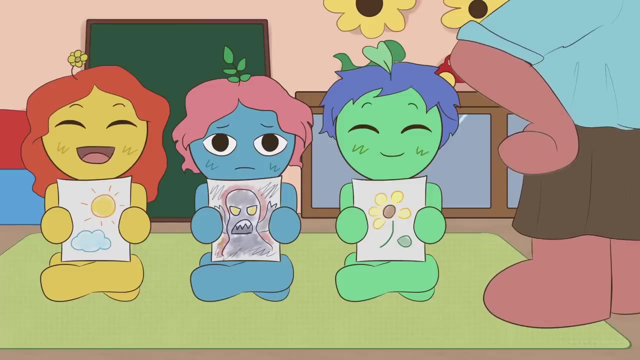 and usually occurs in relationships with abuse, assault, neglect, violence, exploitation or bullying. What does it really mean? Can childhood trauma affect your life as an adult? The answer is yes. Research has shown that adverse childhood experiences are much more common than acknowledged.